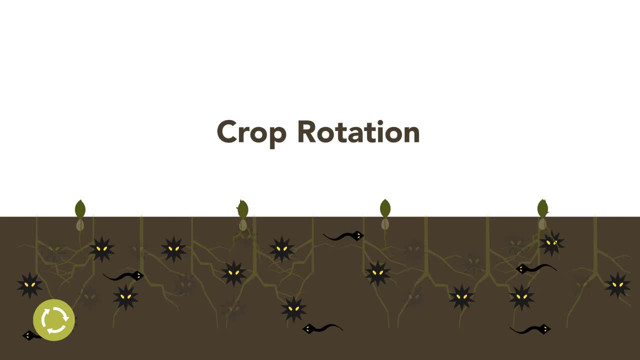 This action harnesses natural factors such as starving of the pathogen or antagonism by beneficial soil microorganisms, meaning that the populations of the pathogens and nematodes will decline to the point that potentially susceptible crops can be grown successfully again in the same soil. 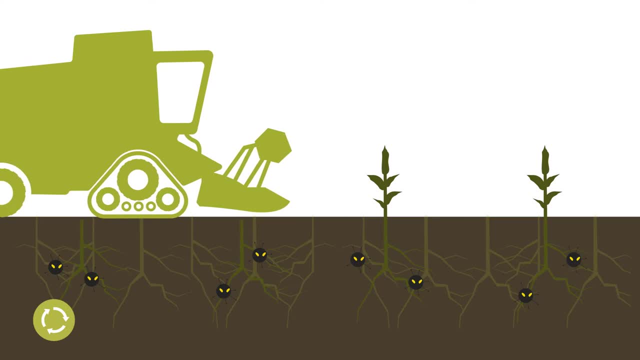 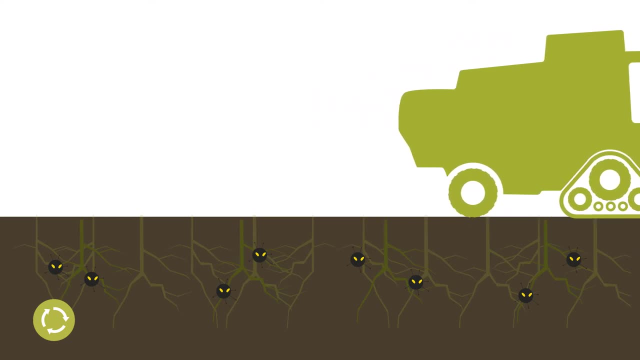 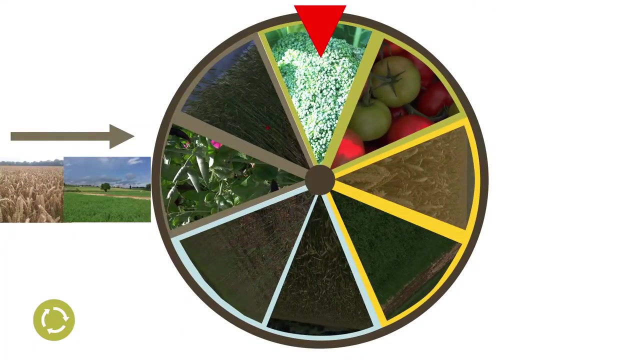 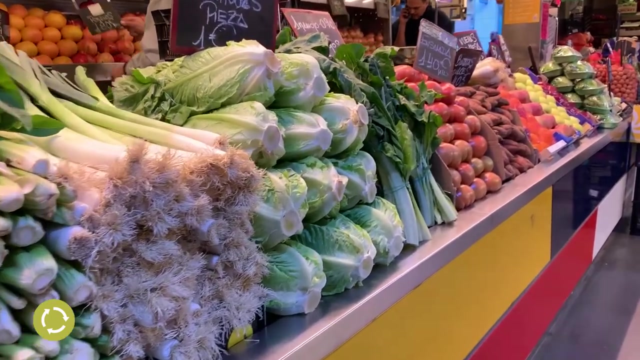 A good crop rotation prevents pests and diseases reaching a population density in which they affect crop yield and quality, resulting in an economic loss for the farmer. It increases or preserves soil health and thus helps to maintain the profitability of the crop. First of all, a sound crop rotation is adapted to the local conditions. 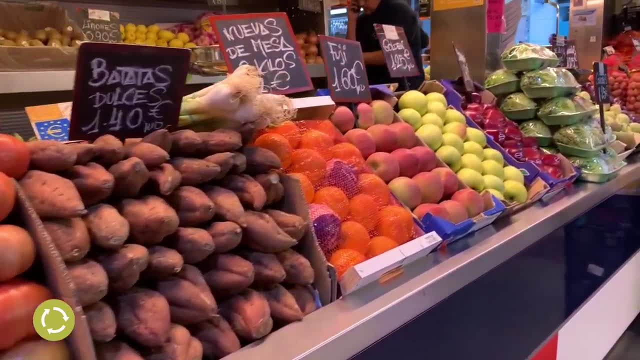 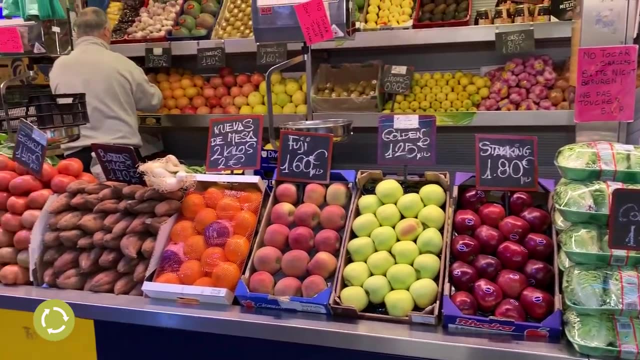 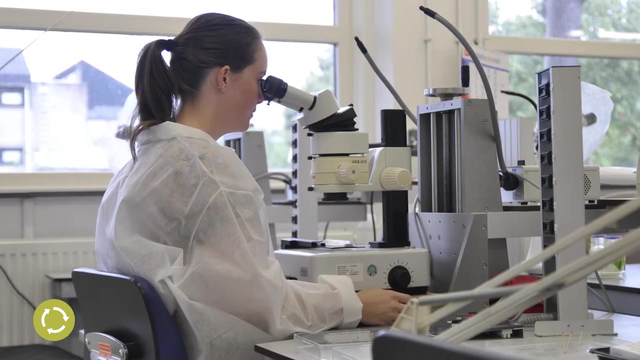 Apart from market opportunities and soil type, the infestation level of already present diseases and pests determines the rotation scheme. Determination of the soil infestation level by nematodes is relatively easy and in many countries public or private laboratories offer such services. 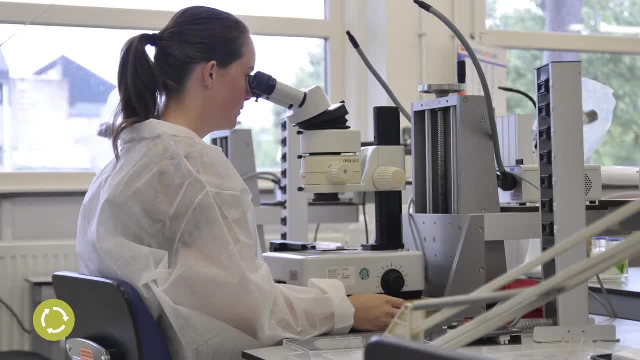 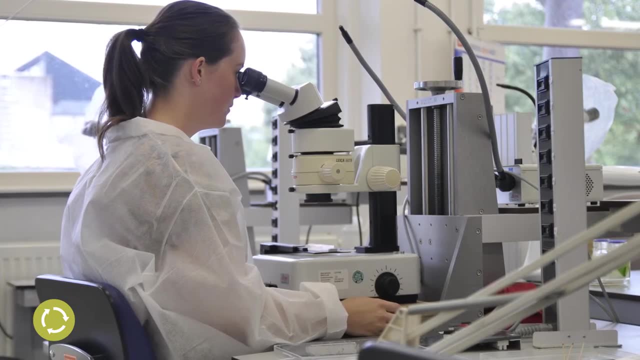 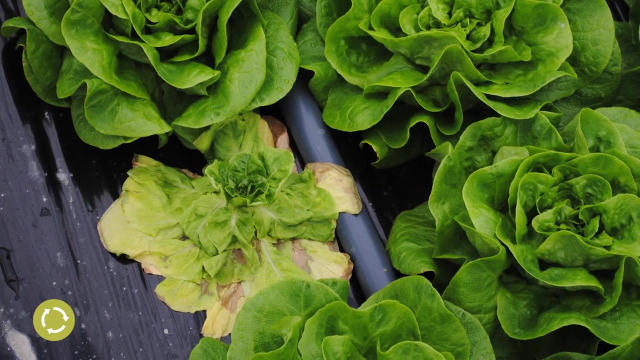 In contrast, only a few of such methods exist for soil-borne fungal pathogens, for example for verticillium, And this analysis is only available in a limited number of countries. Therefore, a sound rotation is especially important to manage fungal soil-borne diseases. The host range for soil-borne diseases and nematodes has to be taken into account. Some diseases and nematodes have a rather narrow host range, for example potato cyst nematodes, while others have a wide host range, such as Trichodorus spp. 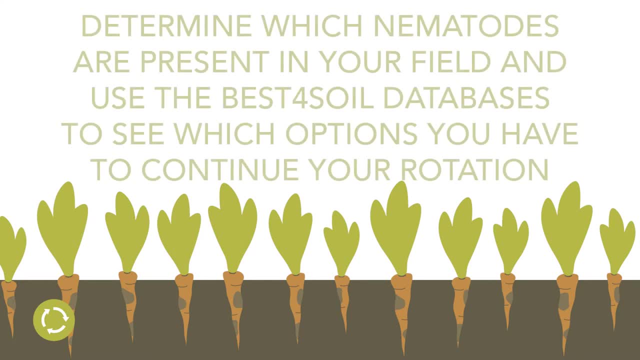 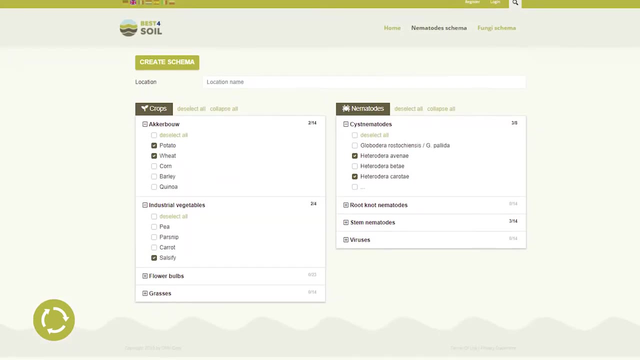 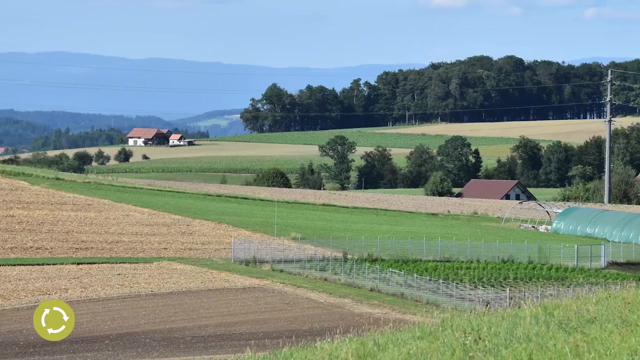 The design of the crop rotation is highly dependent on the crops and which diseases or nematodes are already present in the field. Here we will design a sound crop rotation with the help of the Best for Soil database. One example is a field on a sandy soil in northern Europe. 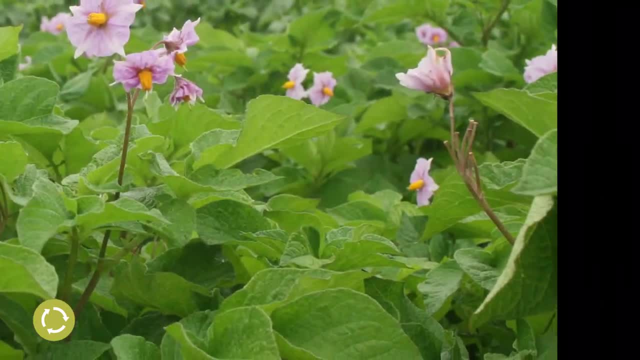 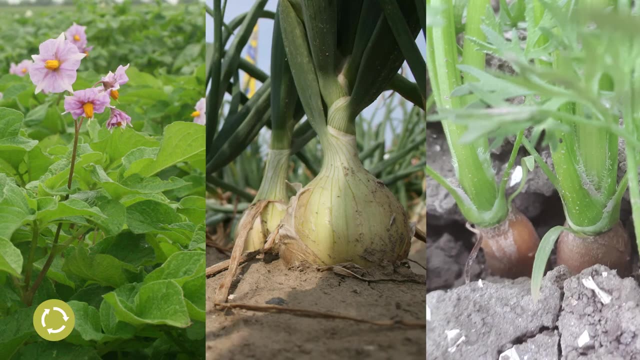 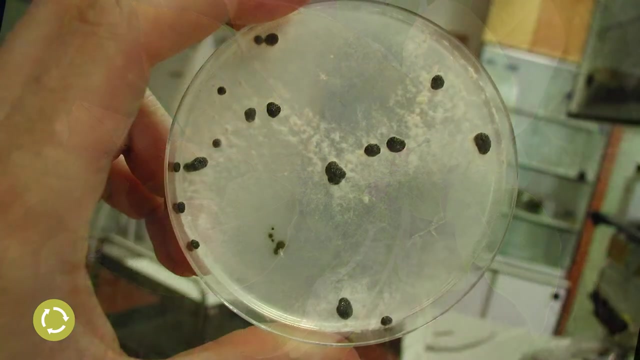 We have a rotation of eight years. The main crops are potato, onion and carrot. Typical soil-borne diseases and nematodes for these crops are Verticillium dahlia, Sclerotinia, sclerotium Fusarium. 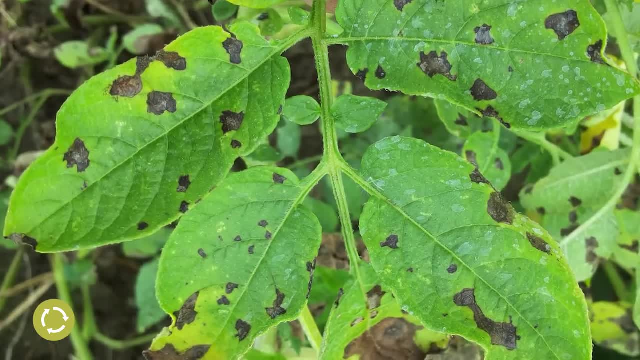 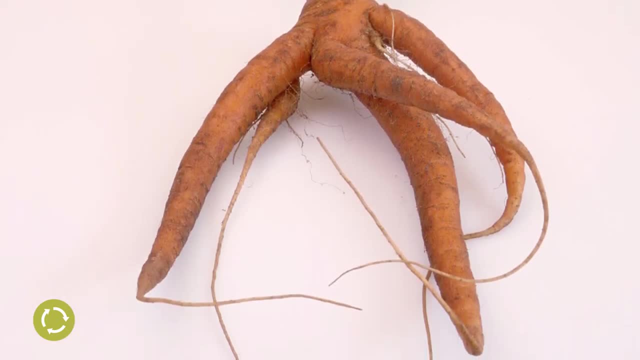 Foma terrestris, Alternaria raditzina, free-living nematodes, the nematodes Pratylencus penetrans and Trichodorus spp. Within this rotation, we grow potato two times and the other crops are sugar beet. 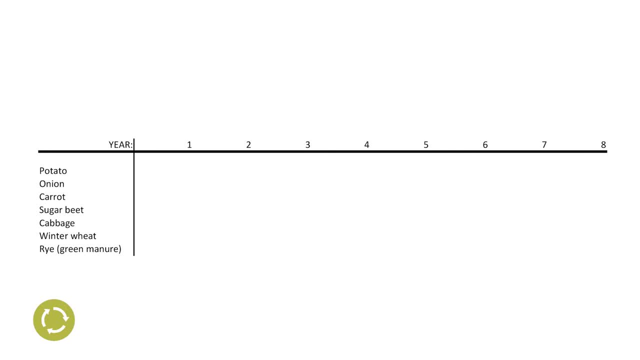 cabbage and winter wheat with rye as green manure crop. A general rule for the frequency is to grow a crop no more than once in the two or more years. For many crops, however, a longer period is required In this rotation, for example, 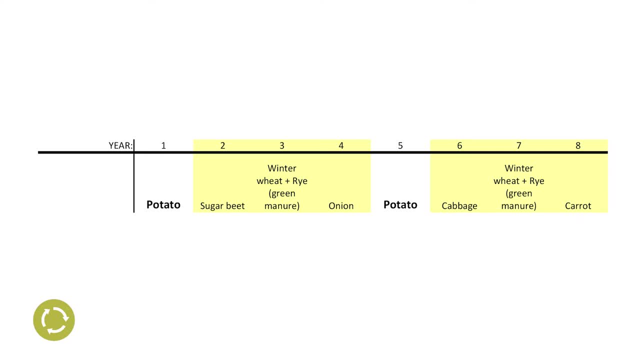 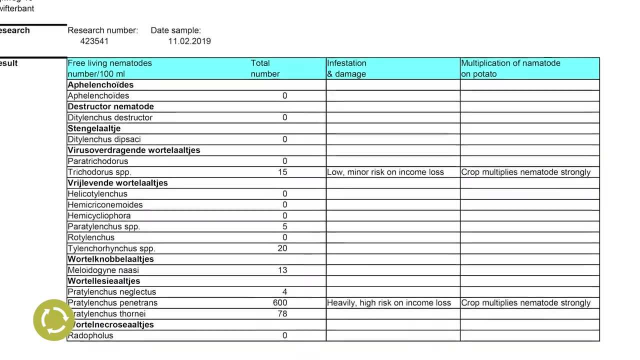 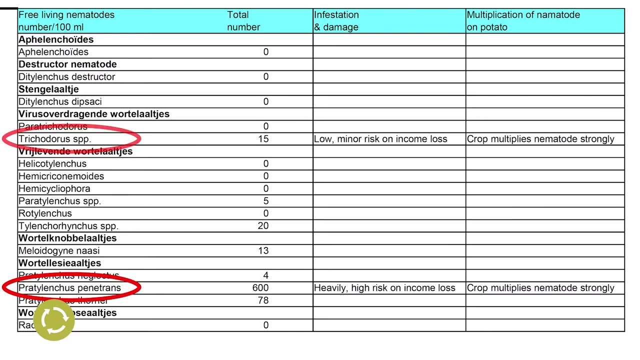 the main crop, potato, is alternated by three sequences of other crops. Soil analysis and observations from previous crops show that the following nematodes are present in the field: The nematode Pratylencus penetrans and the nematode Trichodorus spp. 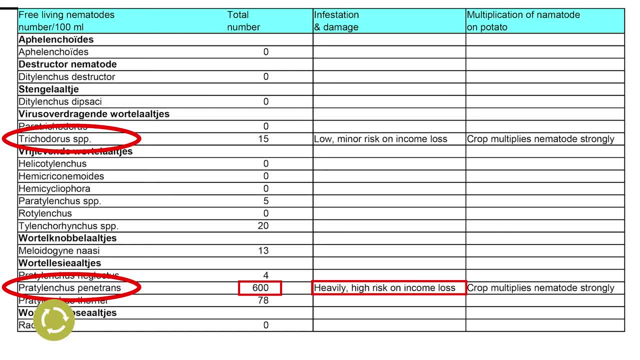 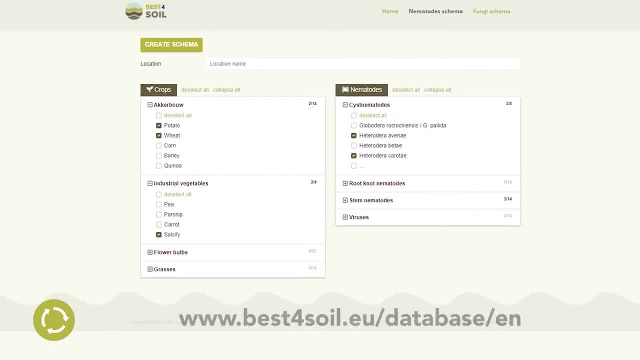 The level of nematode Pratylencus penetrans is above the damage threshold. Therefore, we look into the best-for-soil database to see which non-host plants we can grow After filling in our proposed rotation. the scheme shows at which level. 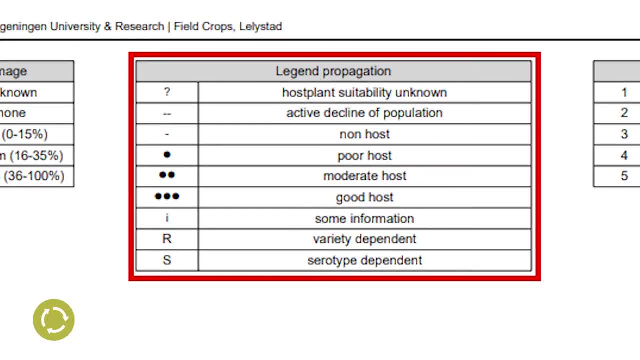 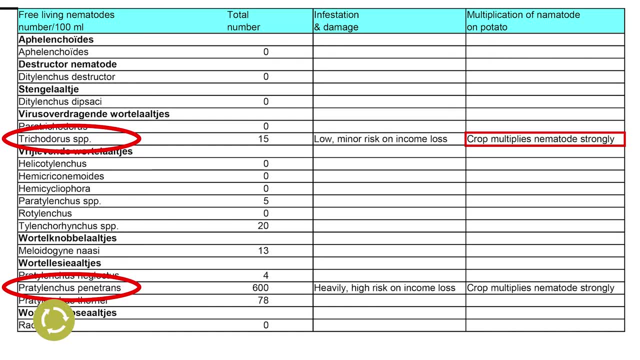 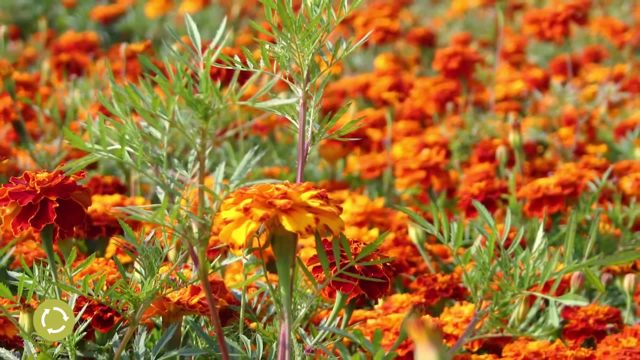 a nematode could multiply on the chosen crops and at which level the crops suffer from the nematode. As we see here, Trichodorus, is not always harmful, but multiplies on all crops. Therefore, we decide to introduce the cover crop Tagetes partula. 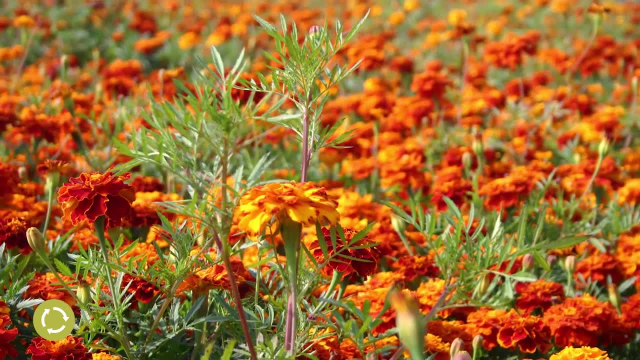 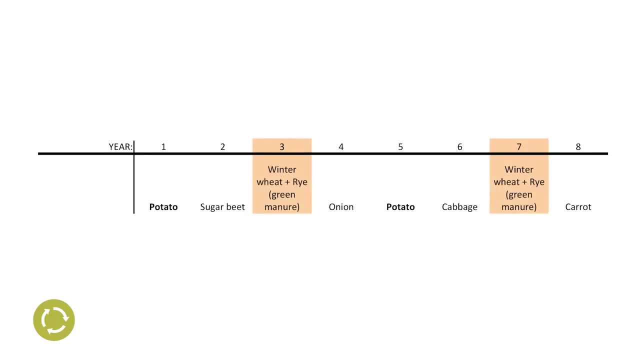 since Tagetes releases a substance deadly for Pratylencus when these nematodes enter the plant. We see that another weakness of our plan is the sequence of winter wheat and the choice for rye, because Pratylencus multiplies strongly on rye. 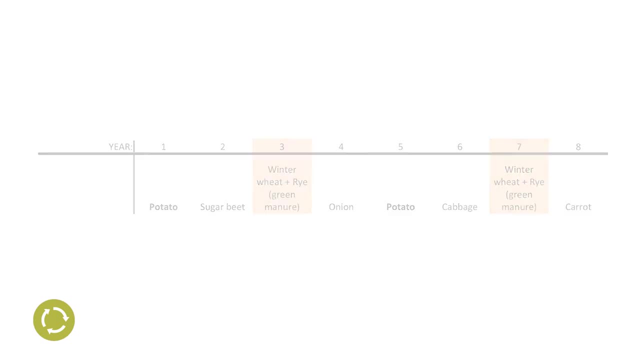 while only a little on sugar beet. Even better options instead of rye are Japanese oat and summer barley. so we decided to switch sugar beet with summer barley and replace rye by Japanese oat and Tagetes as green manures. This is an example of an improved crop rotation.